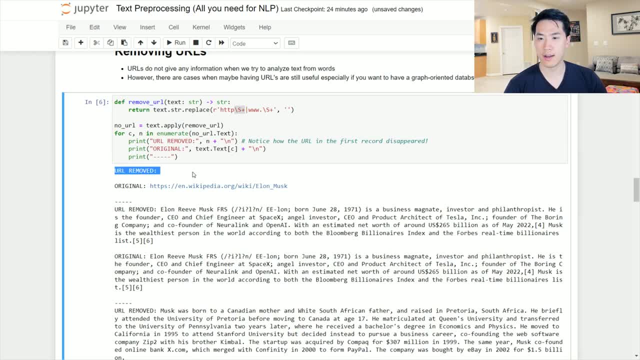 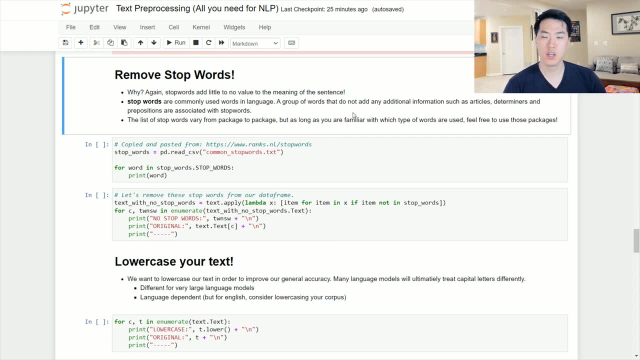 and this is just an example. we only have one url, and so this is our clean text. as we can see, we don't see our https over here, so moving on. so stop words. stop words are essentially just words that don't add any particular value to the actual sentence, and just removing those stop words. 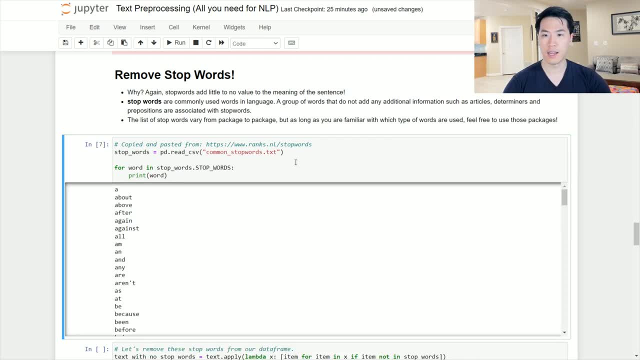 reduces the complexity of your given nlp models. and these are the words, the most common words, i would say, and i just essentially just got this list from this link right here. in general, these are all the words that don't really necessarily add any value, and, of course, you can edit this list. 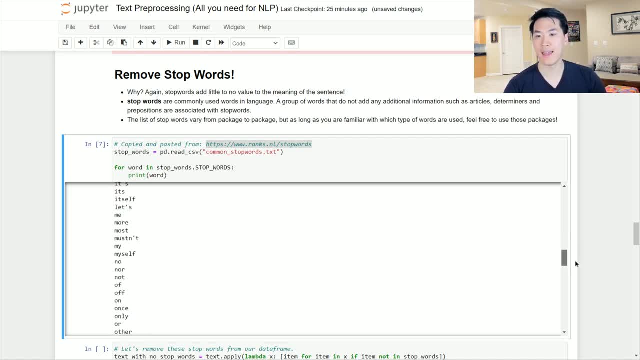 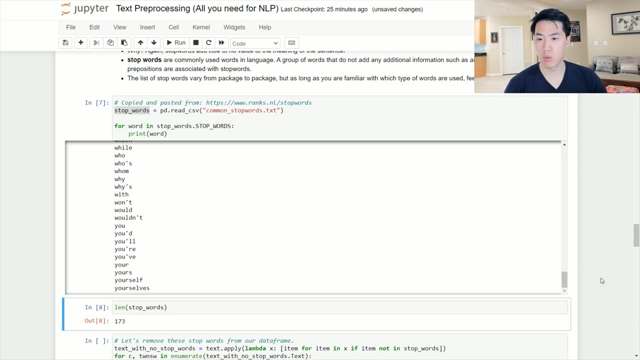 and take out some words that you think add value, and you can even add additional words that you don't think add any value. we have. how many words do we have? we have close to? i think we have like close to. yeah, we have 173 stop words and some other libraries that have like a few hundred more. 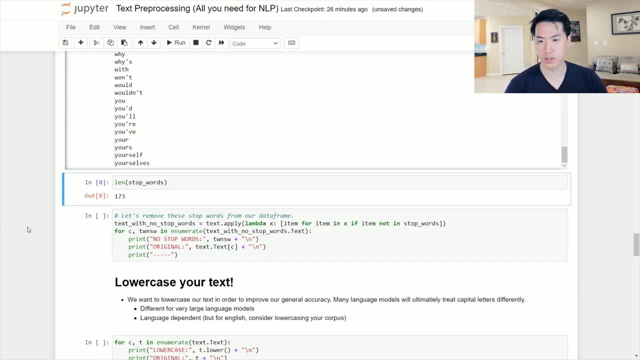 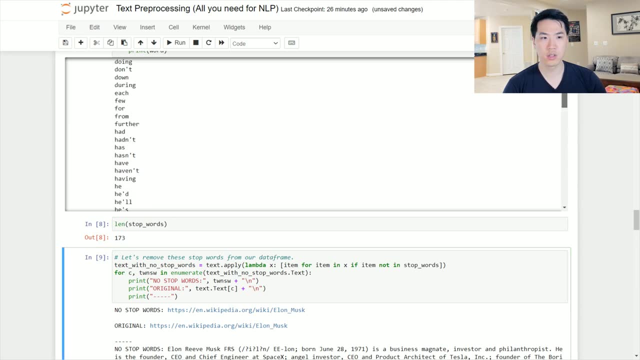 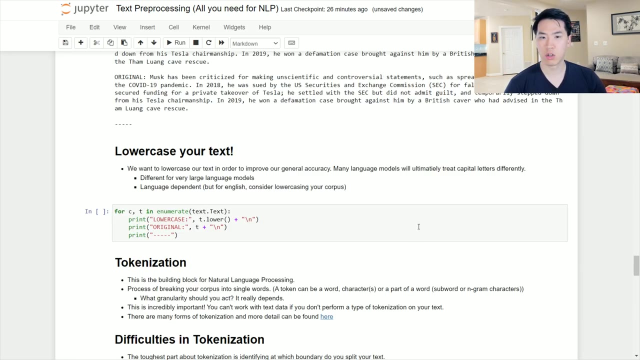 uh, these stop words, but you know you can pick and choose whichever you would want now to remove these stop words. um, yeah, i just wrote like a quickly and the function is iterating through. it's actually just looks throughout this list and looks throughout your strings and just removes those stop words. all right, so next one, lower casing in: 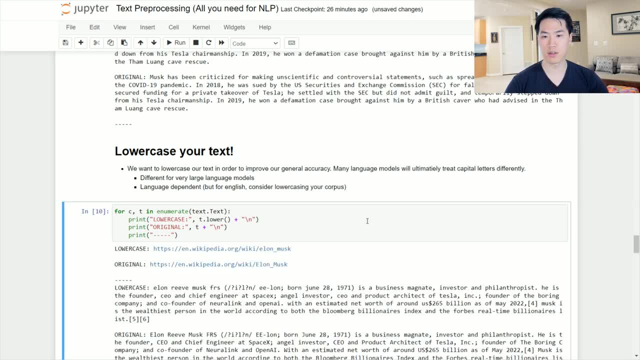 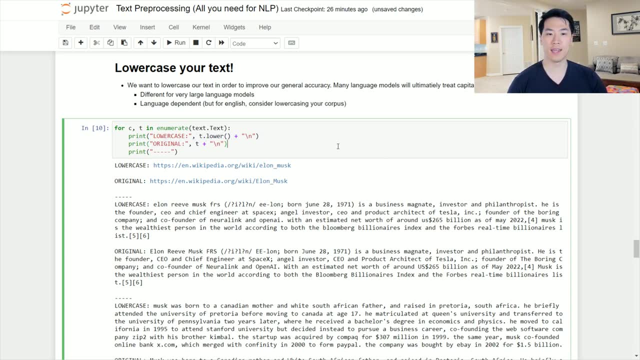 general, it's a good idea perhaps to just lowercase your entire, like all of your text. as we can see, it's just like a really quick function, the to lower function over here, and it just lower cases everything and if it's like a special character, it just leaves it alone, as we can see what's going on. 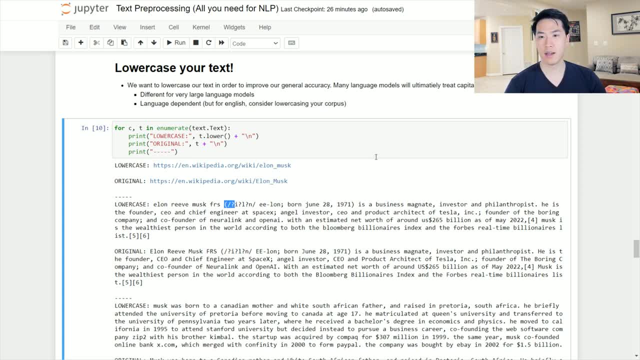 over here. it just leaves those alone. now, the idea behind the lowercase aspect is that many different types of language models are going to have a lot of different types of language models. that are going to have a lot of different types of language models. they'll consider a capital e, for instance. 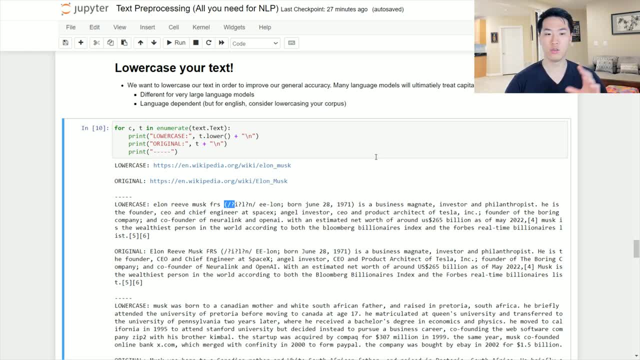 different from the letter, or lowercase e, and it could look at the words, the word embeddings, a little bit differently and hence a different meaning. just so that you are on like the same playing field. you would ideally want to lowercase your text unless you have like a huge, huge model. 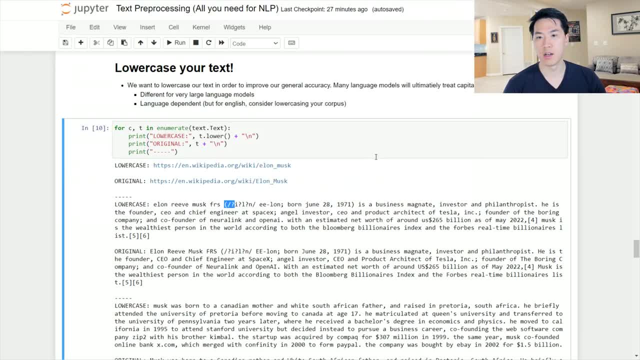 like a gpt3, where it considers both of those particular situations. but in general, when you work with smaller models, you should perhaps lowercase your text, and this is how you would do it. yeah, okay, so next we have tokenization, and so this is an example on what tokenization will look like. 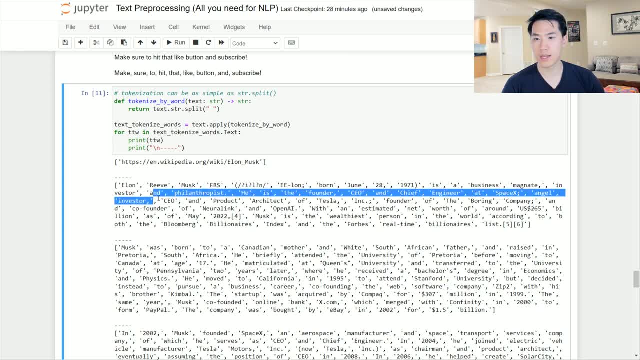 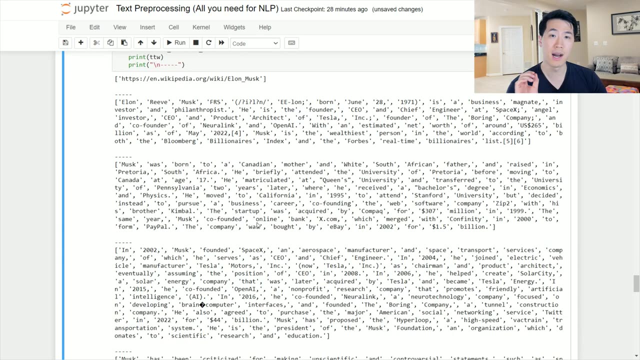 this is the output value, where we have each individual word that's separated by a space is by itself. so elon reeve musk, those are three different words and they're three different tokens. now, tokenization, or the idea of tokenization, doesn't necessarily have to be by word. it can. 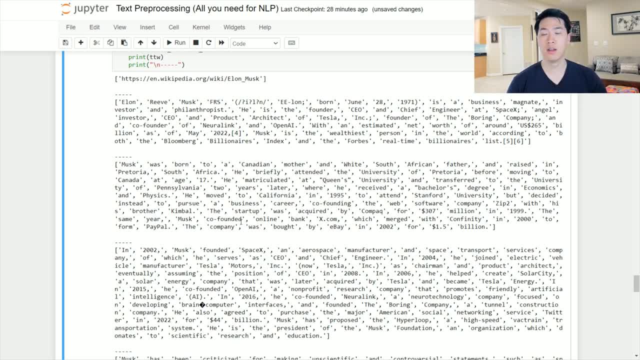 be by like every two characters, every three characters, every two words, so on and so forth, and so forth. so we can see that the more nlp models that you start to play with their back end is a little bit different on how they actually actually pre-process the text. 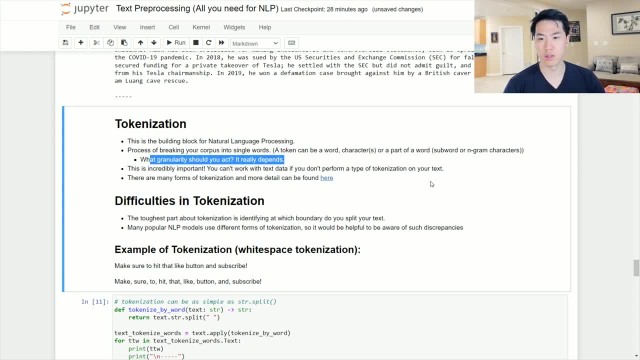 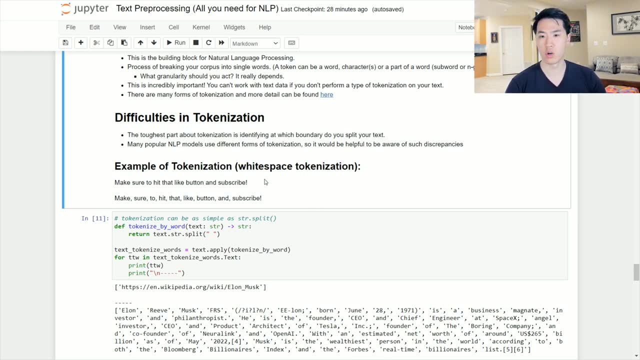 and, of course, we have different types of granularity that you would want to act on. but, uh, just be aware of those differences. they they're not just the um, not just the words themselves. so, for instance, when we have this one sentence, this is just separating it by words. make sure to hit. 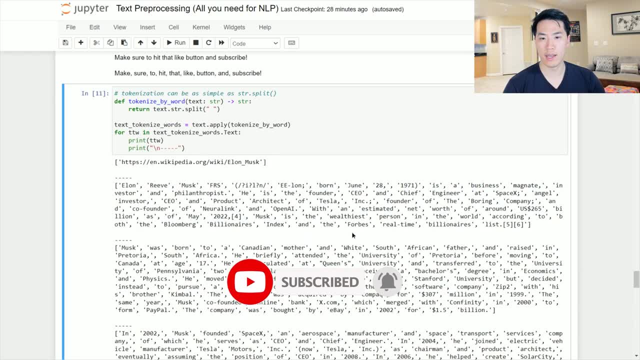 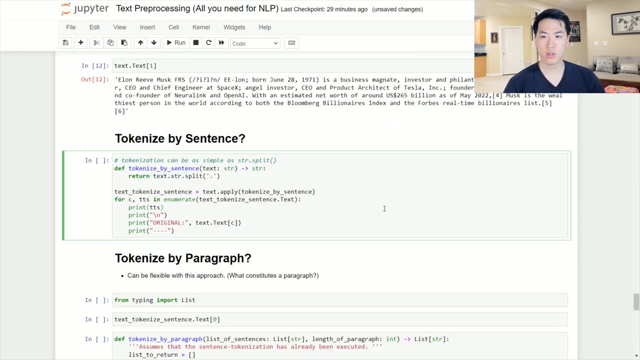 that like button and subscribe and just went ahead and did it by words over here. i also want to point out that this is just an example for our first sentence, but uh, this is also an example if we want to tokenize by sentence. um, it's essentially just looking for those periods and then just 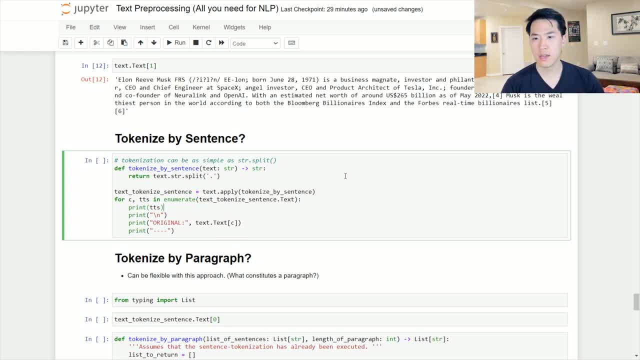 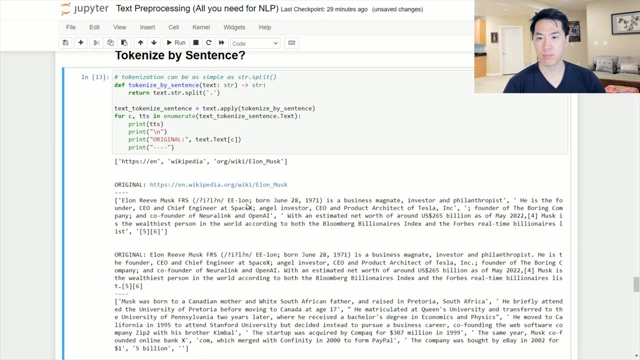 separating or just saying it was splitting their strings based on periods, and i just went ahead and wrote that quick function right there and when we what we have here is just the printed output of each individual sentence looking for that period. so for each one of those commas, those represent 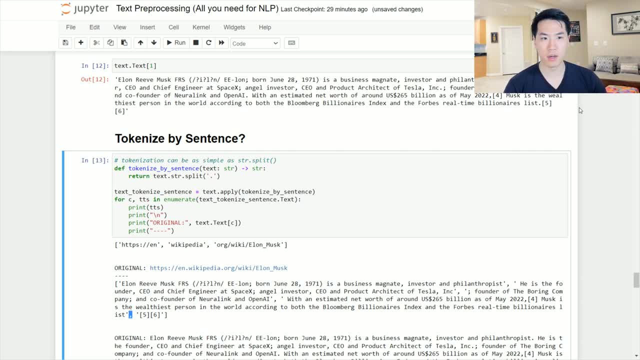 a period because they are separated or split by that period, and then they're separated by that that period. so, as you can see, here we have a period here, and five and six is its own, this own string, and then this is going to go all the way up to here. i think that's the next nope we have. 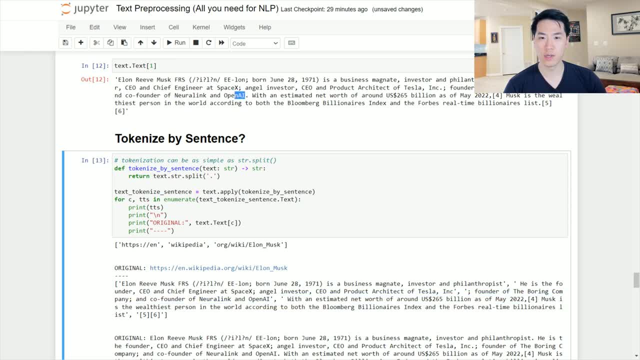 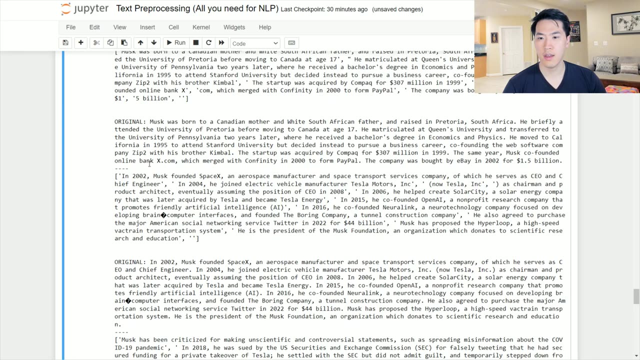 another sentence right here, right before the width, so open a i. there's a period there. so we'll keep on doing that and within the actual array that we have going on, we just conveniently split out our entire string chunk into individual sentences. so that's how you do about sentences. you can also. 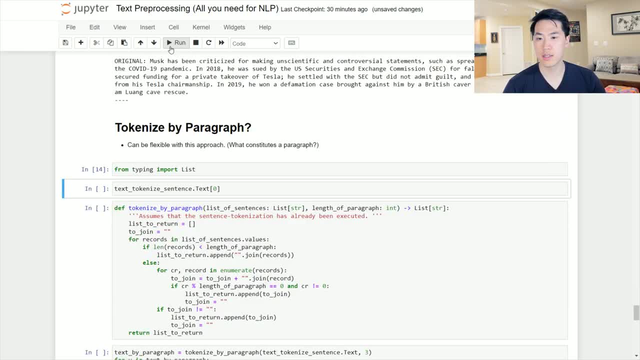 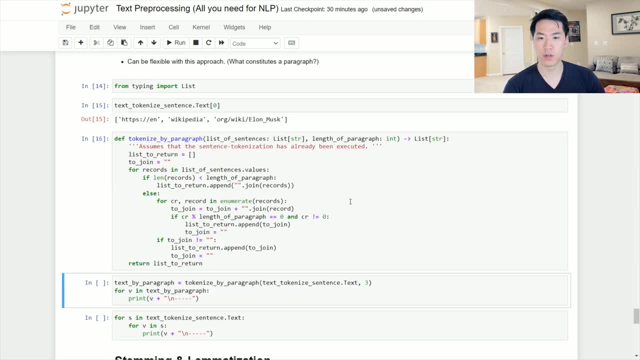 do it by paragraphs, and this was a little bit tricky, um, so it's also somewhat subjective, like you would want to determine what is categorized as a paragraph, and so i just went ahead and wrote this function where it accepts one, two inputs, basically like detailing how long a paragraph. 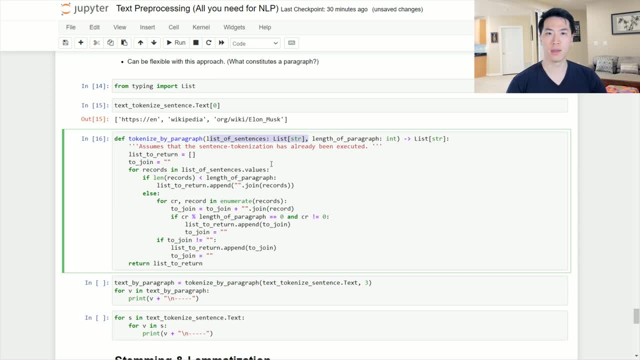 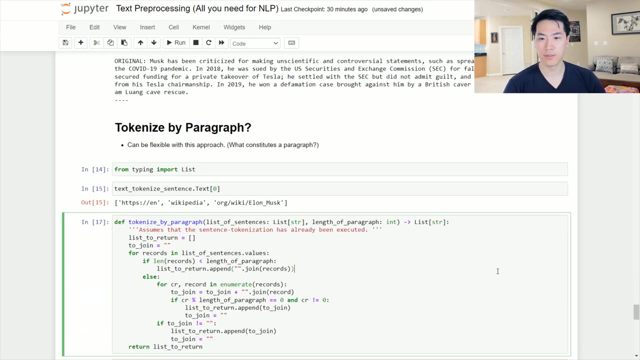 should be, and then the list of sentences that you're going to be inputting into. so, by default, i just said that three sentences will default to a paragraph and it uses the sentences. that sentence eiser function i just created up here and it just essentially just chunks it goes. 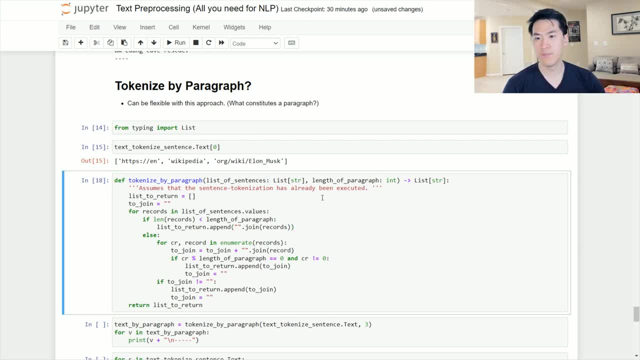 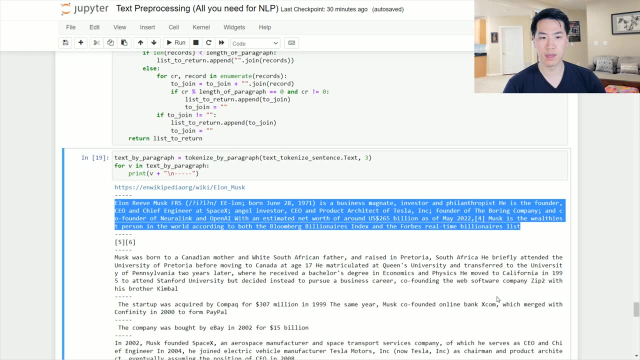 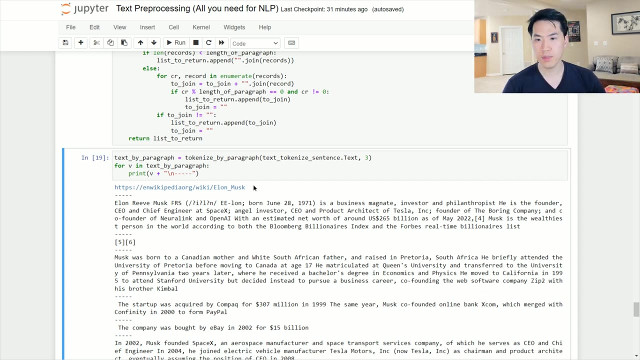 ahead and chunks and it handles those edge cases that we might have. so just run that, and this is what the paragraph chunk idea would be. so the first three sentences would be the you know its own paragraph, and then everything that falls on after it just chunks. chunks it right after and 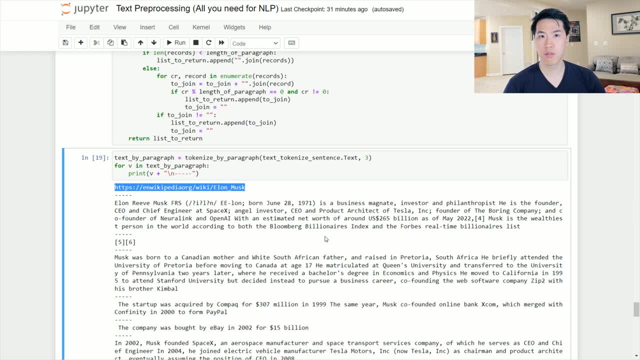 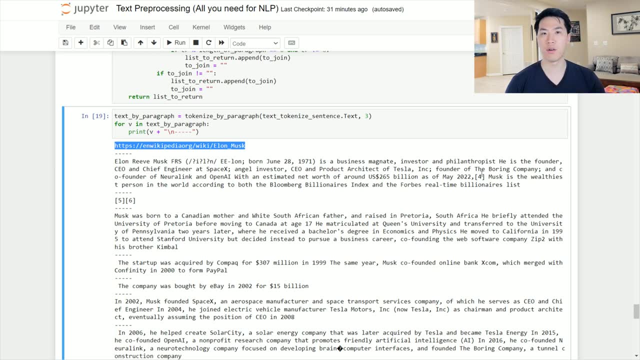 you know, if there are sentences that are less than three in total length, it would, just, you know, return that particular string by itself. so you can perhaps use this for some other nlp models that you might need, or whenever the situation is most convenient when you are trying to tokenize based. 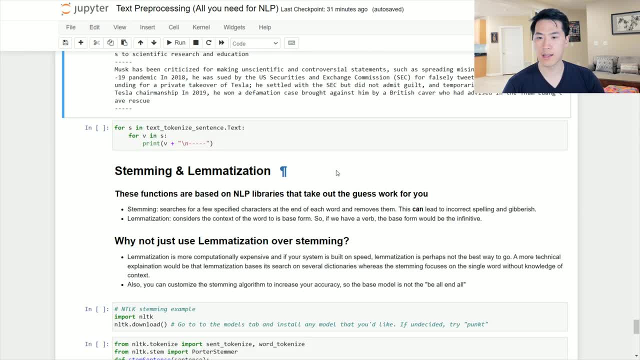 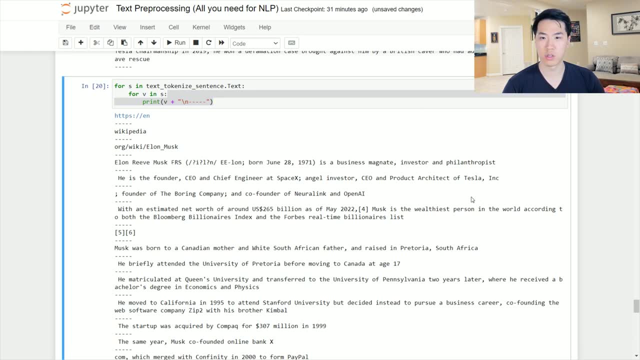 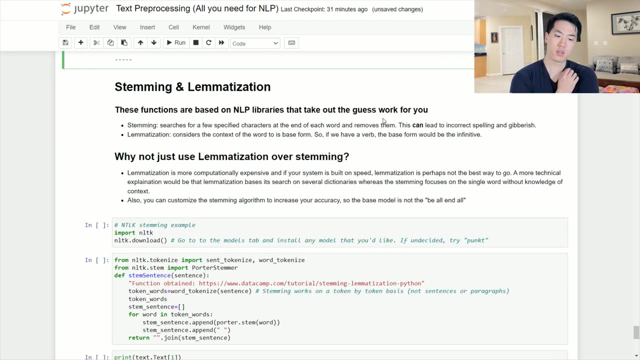 on a paragraph, paragraph formats. so that's how you do that event. and this is last but not least, if you want to see what that token, tokenization by sentence- looks like by each individual one, so that is what that looks like, and now we can go in stemming and lemmatization. so the idea is: 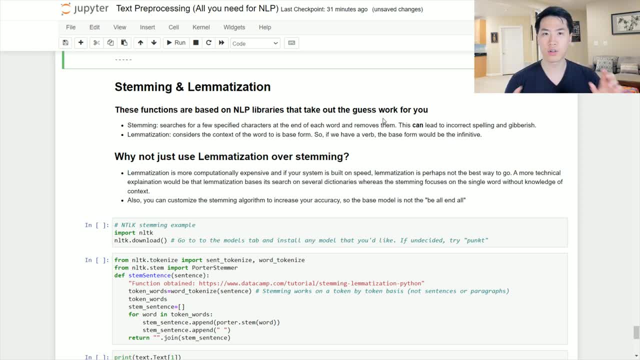 stemming is that it just searches for a key characteristic- um, a key characteristic being a few characters that are at the end of a specific word, and it just chops them off. it does not consider anything related to context or any of that. so sometimes, or more often than not, you can. 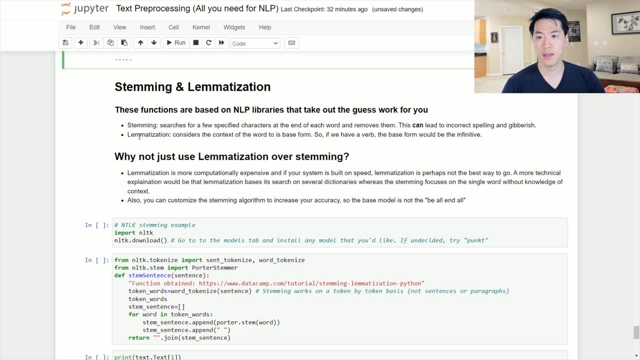 have a lot of gibberish and incorrect spelling. lemmatization considers the context of that word in its base form and it makes more sense when we are going to be lemmatizing a specific verb in that specific context and we won't necessarily have gibberish because all the words are mapped to. 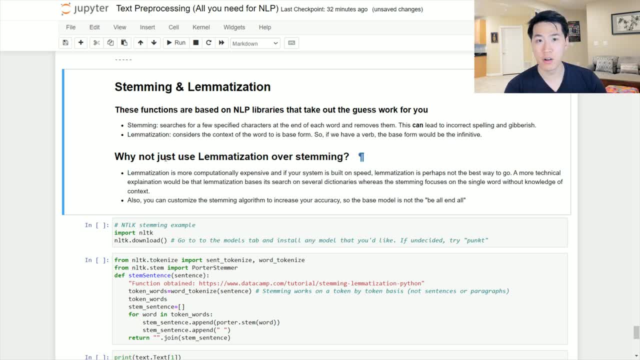 a dictionary, so lemmatization sounds a lot better than stemming, obviously, but there are a few caveats why you would use stemming over limitization, computational power being one. so if your entire system, if your entire base, is built on speed, then perhaps lemmatization is not the best. and another caveat to using, uh, stemming over. 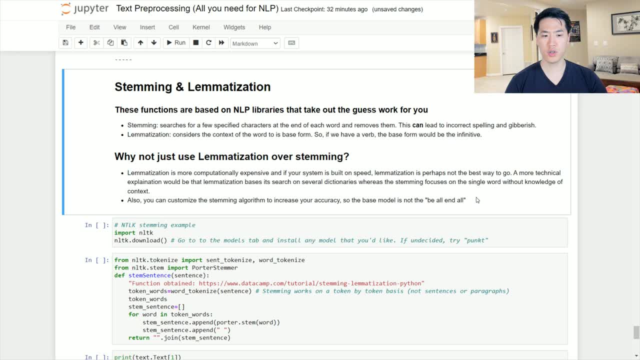 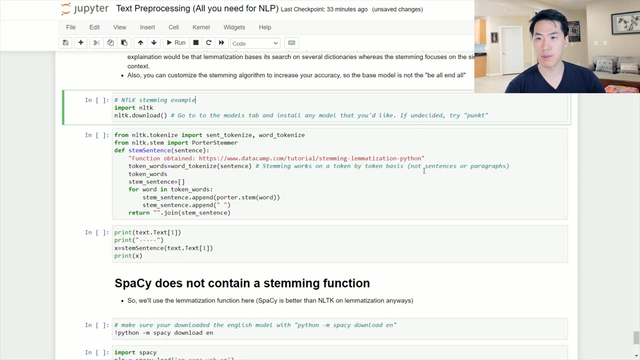 lemmatization is that stemming. you could incorporate some additional rules to improve its accuracy. so if you want to go through the speed route, then maybe researching stemming is probably the best bet. oops, let's try and run that so okay, so i'll be utilizing nltk and spacey. 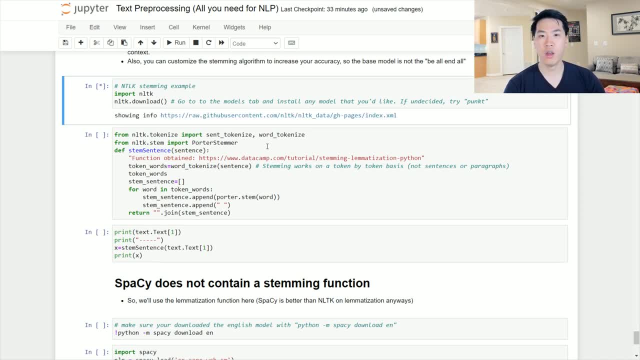 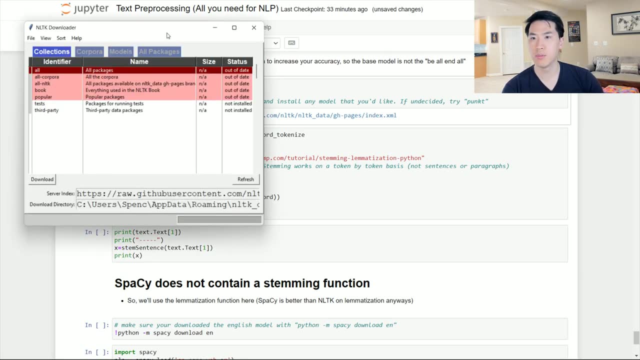 so the nltk. i'll just be going through an example on what the actual stemming process looks like. and i just went ahead and ran this and this pops up on my screen and you just go ahead and click on the model section and i just went ahead and downloaded. 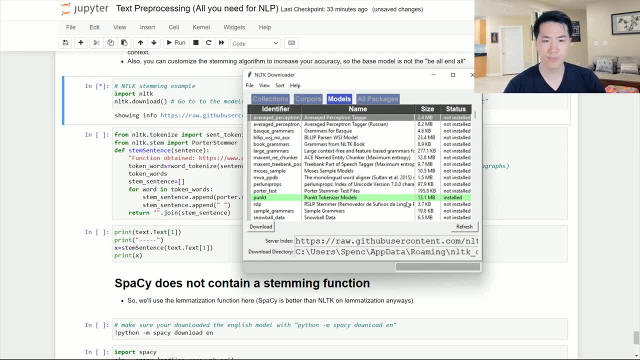 this identifier the punked tokenizer models. it just has all of your associated, i guess, like really small base models that you can go ahead and use. you can also look at the where's the other model, moses sample model, so you can also perhaps use that. but yeah, you can choose any one of those. 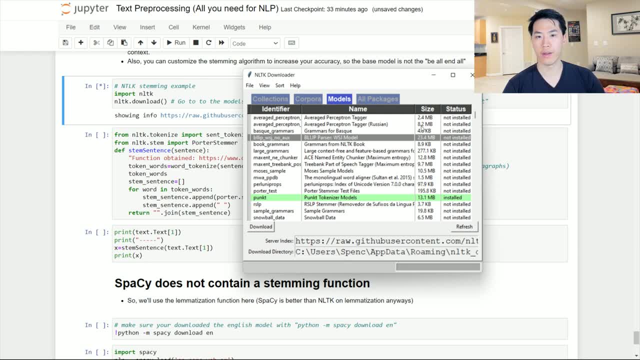 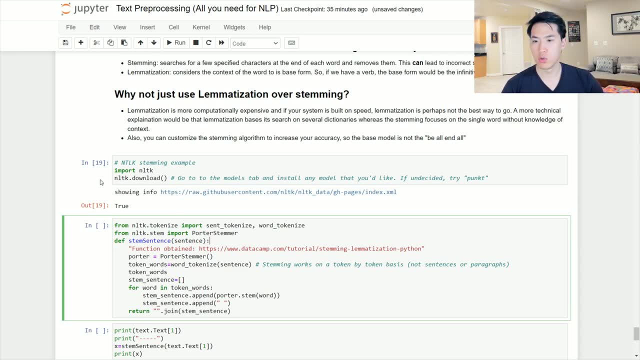 models. anything that has the word model model in it. you can go ahead and check that one out. so i just went ahead and downloaded punked and after you downloaded whichever model that you chose, you can go ahead and check out this particular link on stemming and lemmatization. but essentially, 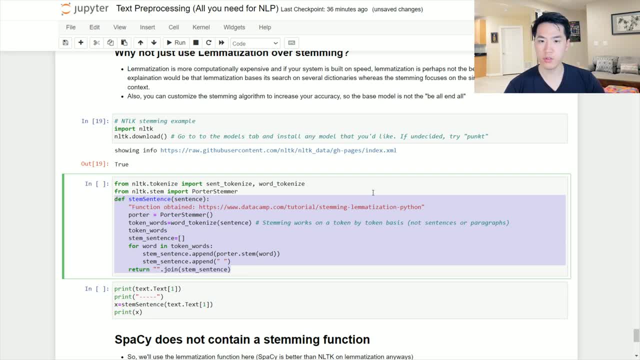 i got this function from that particular link and all it's doing is that it's just splitting, uh, this particular sentence into its individual token and then running the stemmer on top of each one of the words within the list. so that's what that is doing. we can go ahead and run this and. 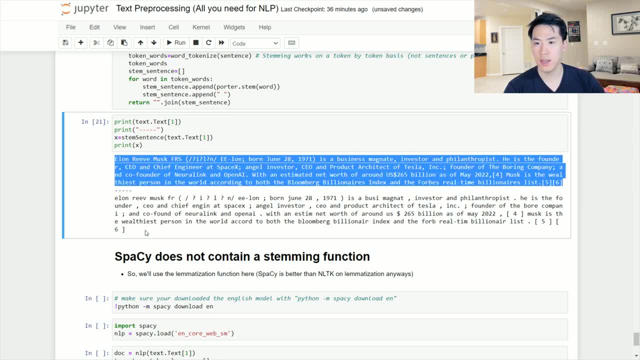 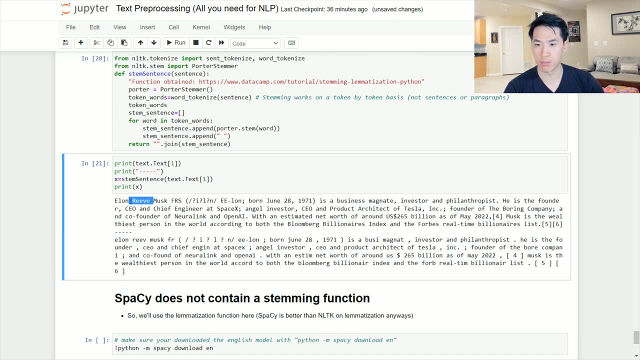 this is the original sentence, or the paragraph, i should say, and this is the follow-on, so, as we can see, stemming could return: gibberish like reeve. there's no e in there, even though this is like a pronoun. uh, we have, let's see what else, what else? 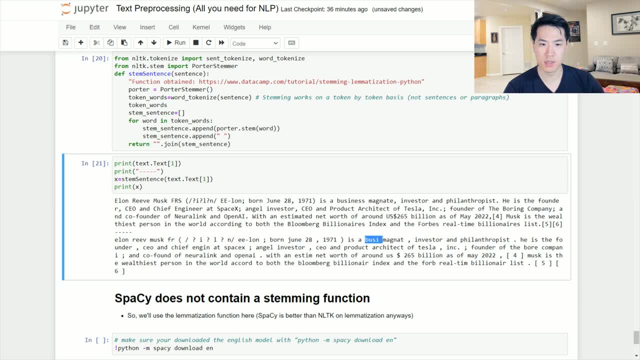 is is: um, let's see business, business, yep. so it just chops off some of those characters that are not entirely relevant, and the main reason why this is happening behind the stemming approach is that stemming has like a list of words, uh, that it looks at and it just automatically stems a particular word to that base root: um, without any. 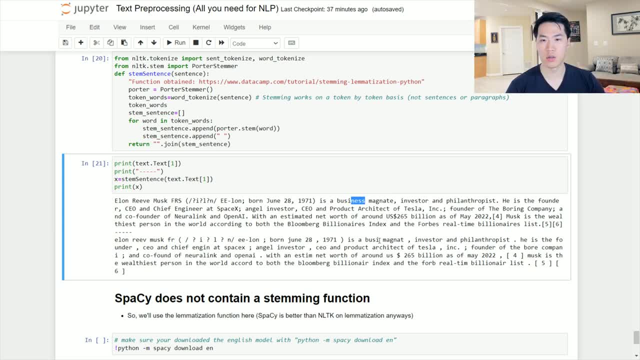 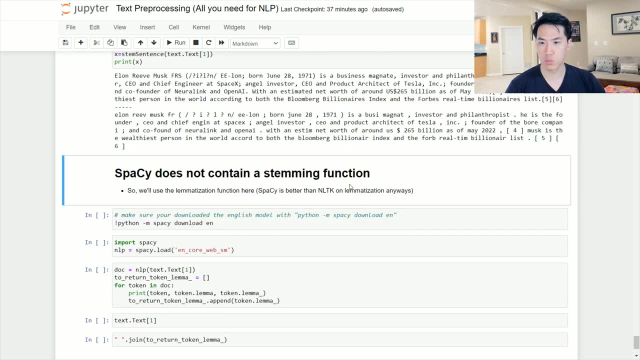 of that context held. so that is why that is doing it and that's why it's a little bit faster than the lemmatization route, where it's basically like lots of dictionaries, and so this is where the spaCy comes in, where it's actually really really well known that lemmatization with spaCy 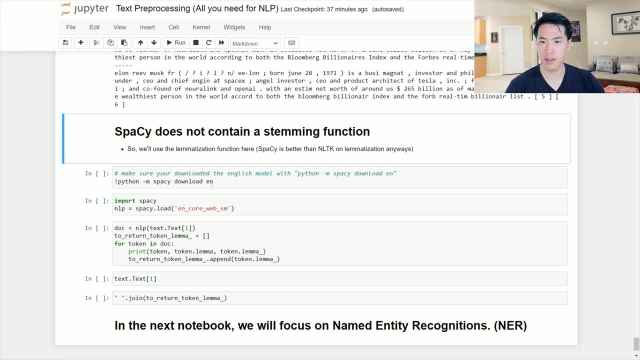 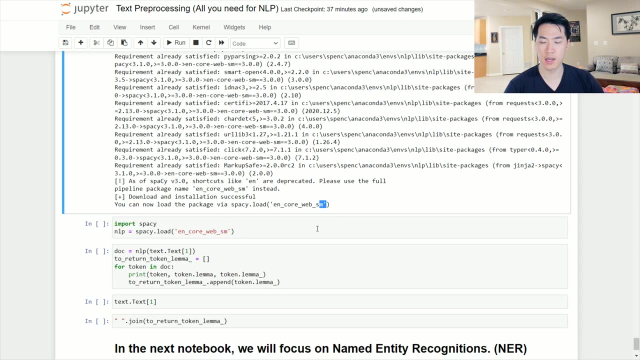 is vastly superior compared to NLTK. um, yeah, let's go ahead and download a basic uh spaCy model in english with the, the en, and it has been downloaded over here and it's a small model sm. is this small so we can go ahead and import that? and, uh, what this is doing is that. 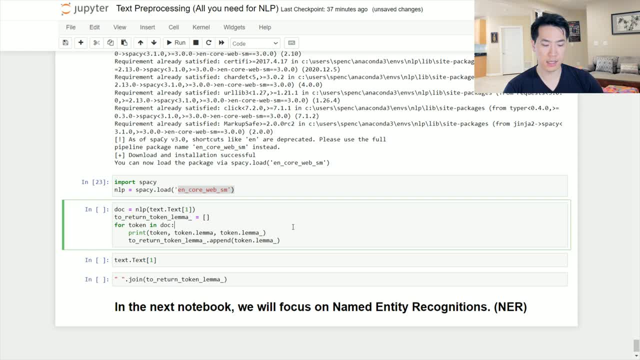 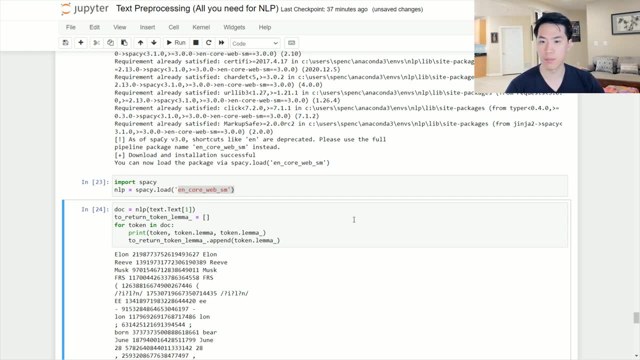 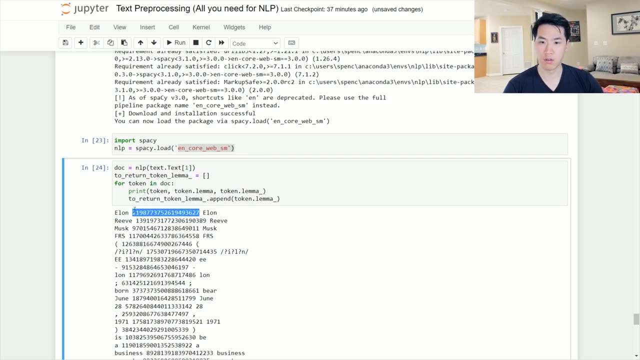 this is already a very small language model in english and it already has a vocabulary on which all of these you know words are matched with something. so what i'm over doing over here is that i'm just printing the original words and i'm going to go ahead and import the original words and i'm going to go ahead and import the 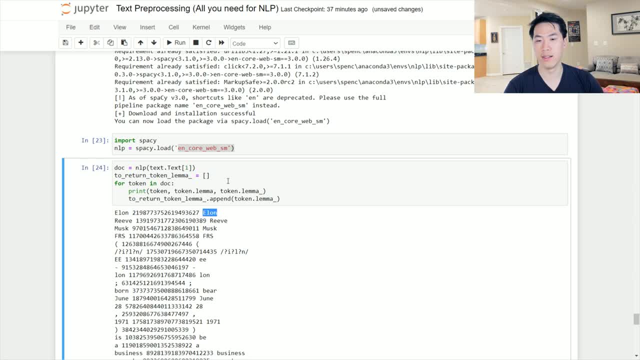 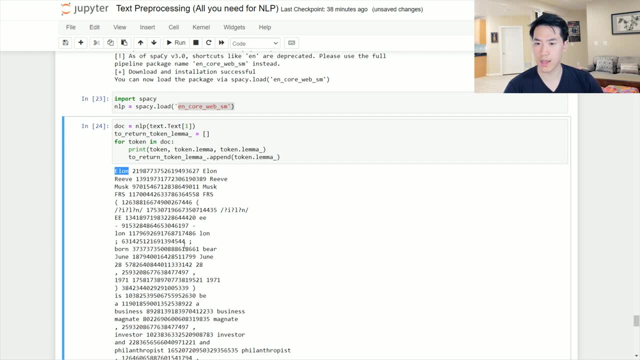 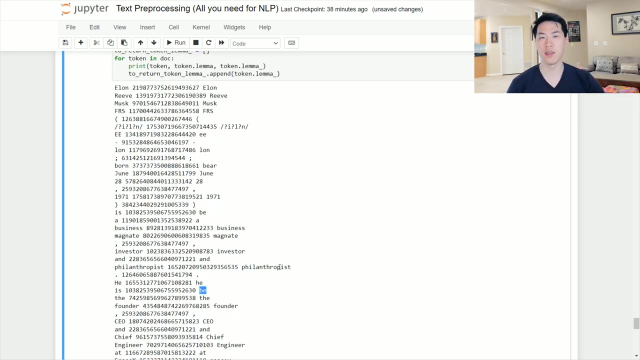 uh, the vector value in the vector space and then the actual lemmatization of the original value. so if we just scroll down here, there's one value i want to point out. if we have the word is, the root is b. so that's what's happening here and that's where the lemmatization is very, very. 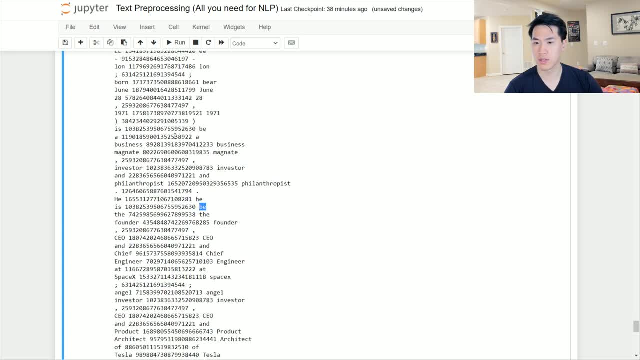 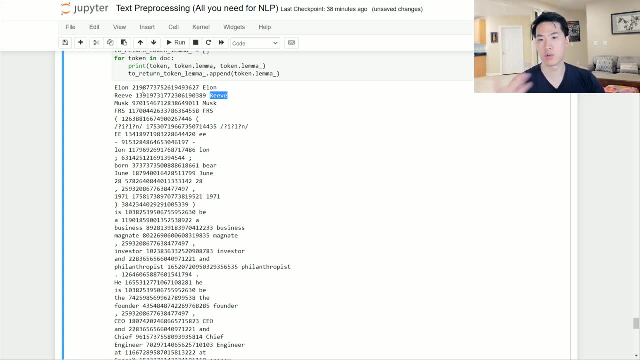 powerful and you can get some really nifty and accurate results. uh, and, as we can see, let's see it here in this particular case, it's pretty simple. so, first of all, let's say we have to print out the original and also the- uh, the joined list of all the lemmatization aspects, and this is what we.